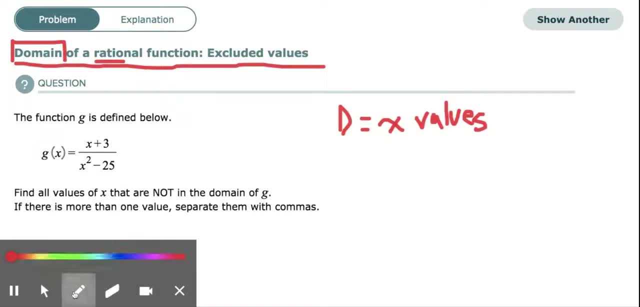 are some excluded values of x, meaning it can't be an x value. Now, what you want to focus on, when you're focusing on a rational function, is the denominator, Because you can have any value for a fraction, but what the bottom cannot be is this: cannot, this cannot be equal. 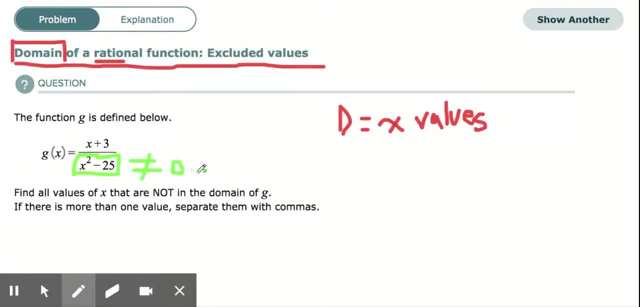 to zero, because you can't divide by zero or else your function is undefined. That means it wouldn't exist if this was equal to zero. So, in order to find all the x values that are not in the domain of g, what you have to do is you have to figure out when would the denominator be equal to zero? 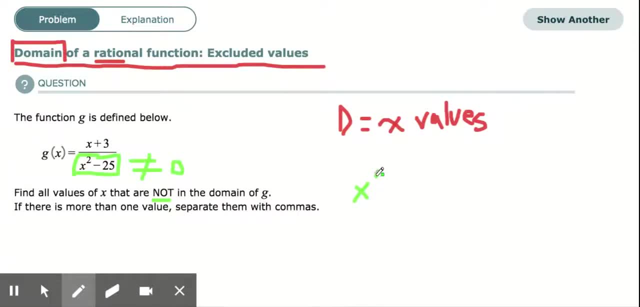 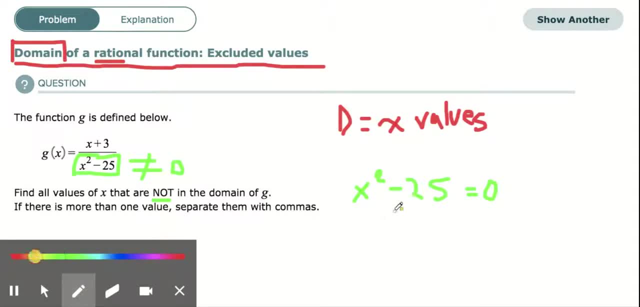 Let's solve for x. In order to get x by itself, you want to add 25 to both sides. Now you have x squared. isolated, x squared equals 25.. And in order to undo a square, you do the square root. That's the inverse operation. So whatever you do to one side, you do to the other. 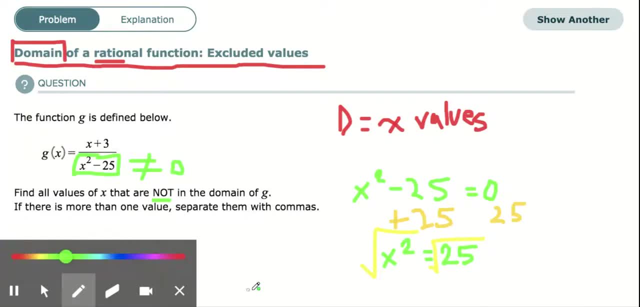 side. Now the square and the square are the same. So you do, the square and the square are the same. The square root will cancel out. So x will be by itself. Now a square root asks us what number times itself makes what's called the radicand, the number inside of the square root. So what? 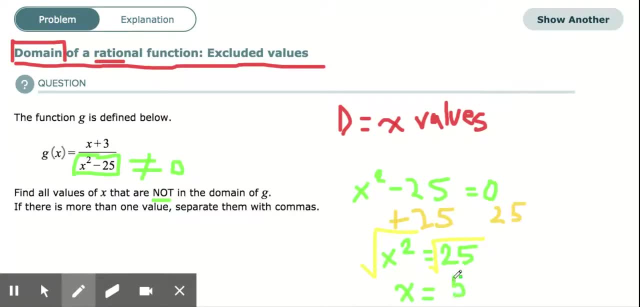 number times itself makes 25?? Well, that number is 5.. However, there's another number that actually satisfies that too, And that number is negative 5, because negative 5 times negative 5 is also positive 25. So we write this as plus or minus 5.. However, this is a positive 25.. So we write this as: 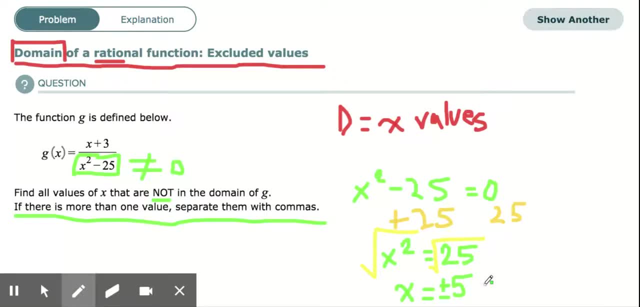 minus 5.. However, this is asking us to write them separated with commas. So, since it's asking us to separate them with commas, since there's more than one value, our answer would be 5 and then also negative 5.. And it shouldn't matter the order that we write those in. Let's check. 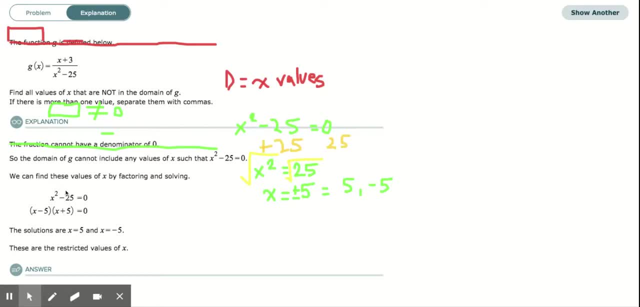 And yes, they factor it down a little bit differently, But you can see that they get the same values of positive 5 and negative 5..